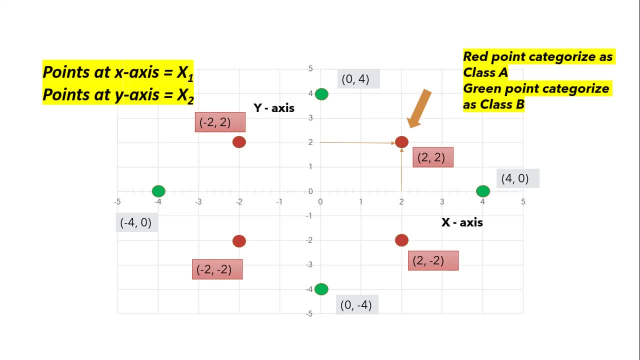 this data in higher dimension so that we can create separable hyperplane between these classes. we will find out a non-linear mapping function, that is phi, through which we can transfer this data into new feature space, And thus we will be able to create separating. 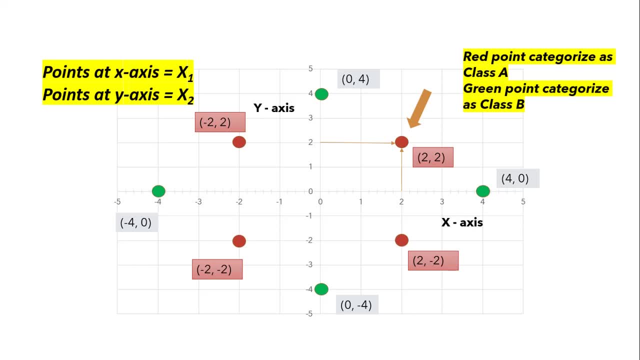 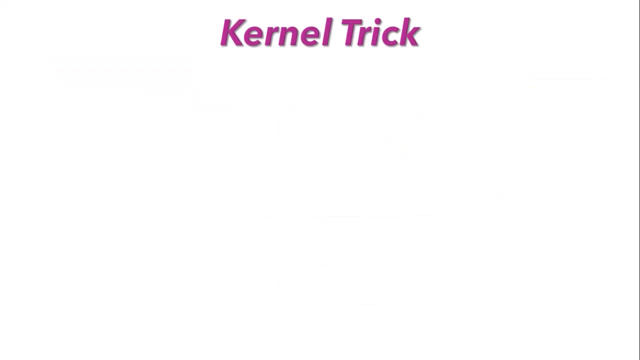 hyperplane. Now questions arises: How can we get this phi value? So what is this phi value? Let's quickly jumps into the video起, jump into kernel trade. So the linear classifier only depends on dot products. So let's define some function ker of point x1 and x2 as just being the dot products. and if I map a data point, 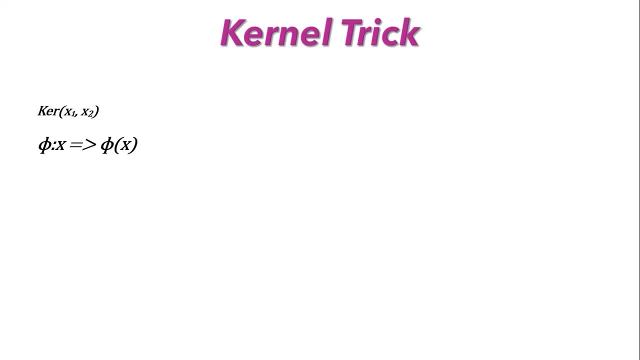 to some higher dimensional space. so my function, phi, will be mapped to x, to phi of x. So the dot product of ker of x1, x2 would become phi of x1, transpose into phi of x2.. So here ker is the similarity function that corresponds to an inner product of higher dimensional space. So, guys, if 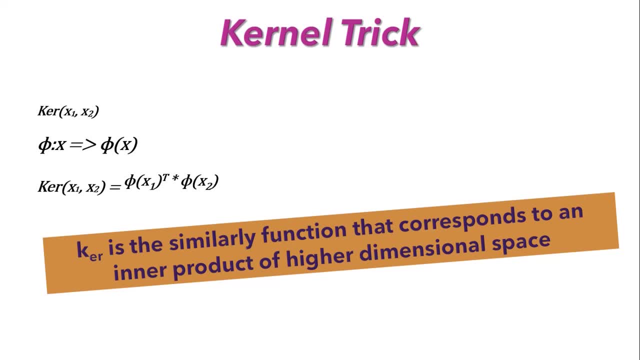 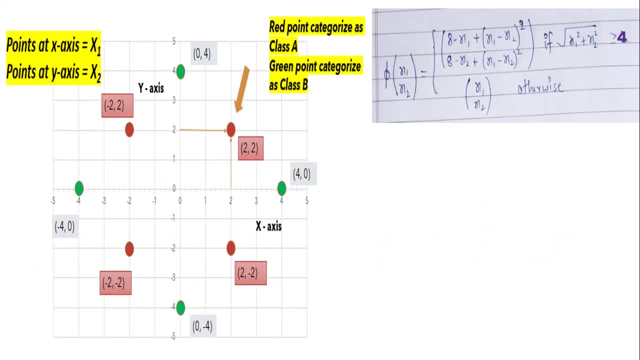 you haven't understood this, then it's not a problem. We will understand this through an example where we can mathematically solve our problem. Now let's say we have a mapping function as shown on the screen, and if we map it to x1- x2, then it will be the dot product of ker of x1- x2.. So we 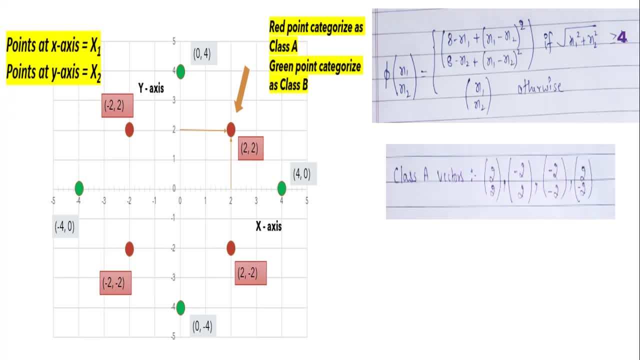 look into class A, then we can find out that under root of x1 square plus x2 square is less than or equal to 4. So there will not be any transformation. but if you see class B, then this will be transformed into different space because the value of under root of x1 square plus x2 square for 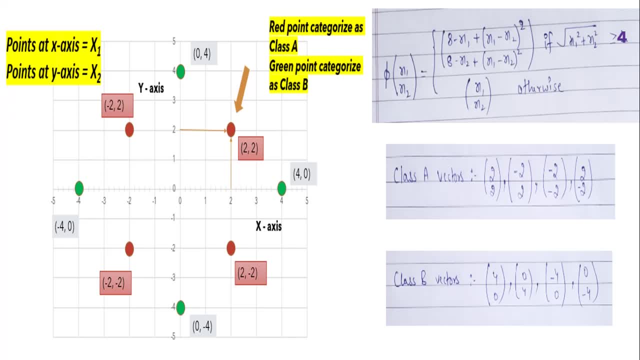 class B is greater than or equal to 4.. Just to add one thing: that under root of x1 square plus x2 square is less than or equal to 4.. So if we look into class A, then we can find out that x2 square is nothing but the euclidean distance. Let's apply this function to class B, So first. 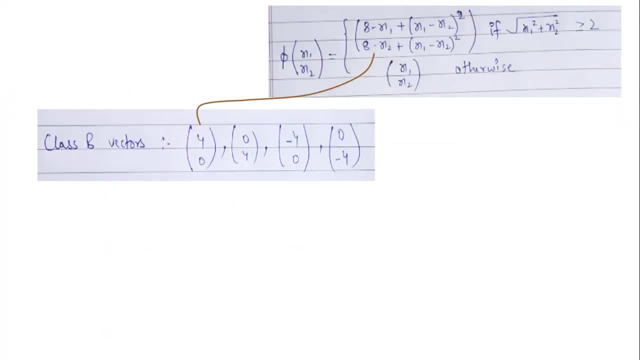 vector is 4 comma 0, and if we substitute x1 as 4 and x2 as 0 in the function, then our phi will be 20 to 24.. Now we have transformed this vector from original vector 4 to 0 to new vector position.